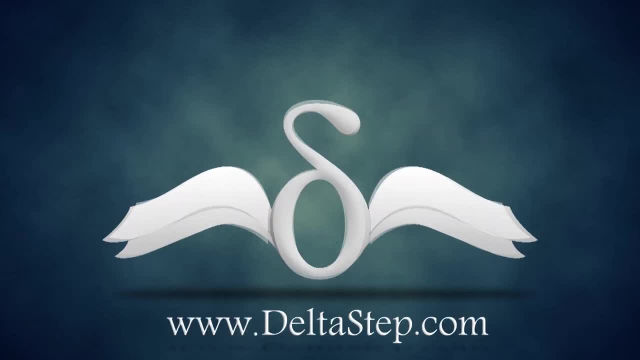 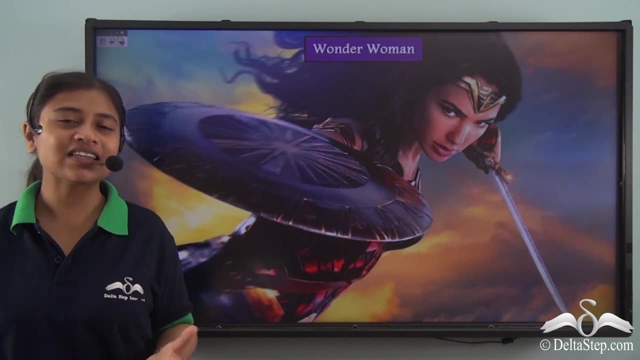 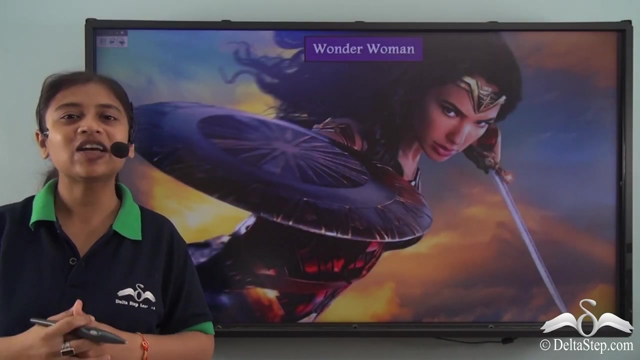 We have always heard about and been fantasizing about superheroes- Batman, Superman, Spiderman and many more- But have you all heard of her? She is Wonder Woman. We all have seen her in movies and comics. Well, she is one of the first female superheroes to be created. 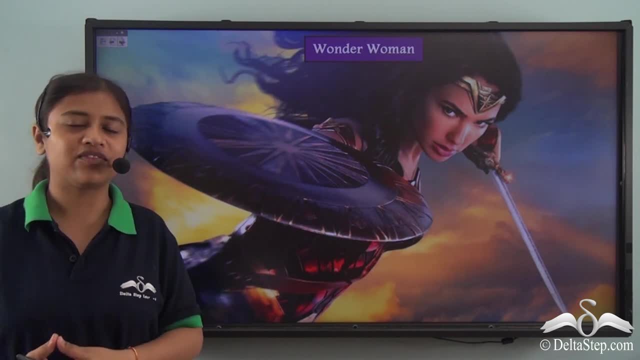 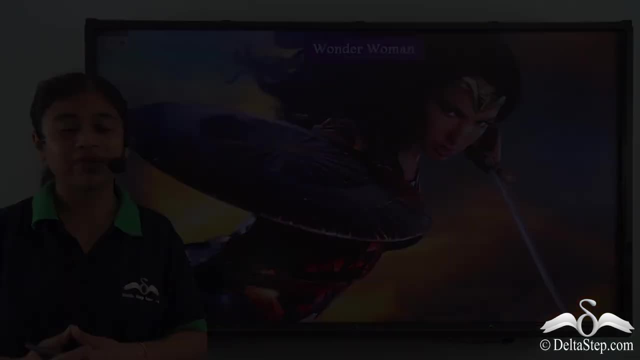 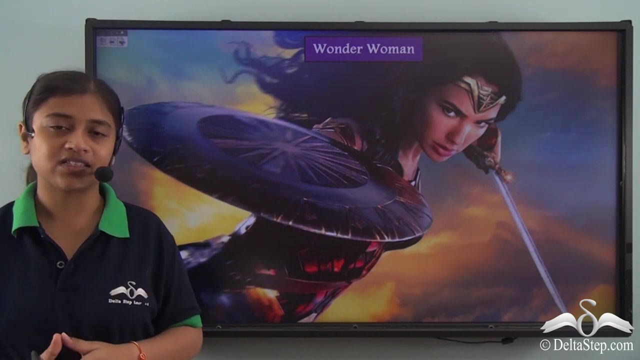 in history and in comics. We all love her, And if you haven't watched her movie, then you must. But why are we suddenly talking about the Wonder Woman? The first thing that crosses our mind is the Amazon, As we all know that the Wonder Woman is the princess. 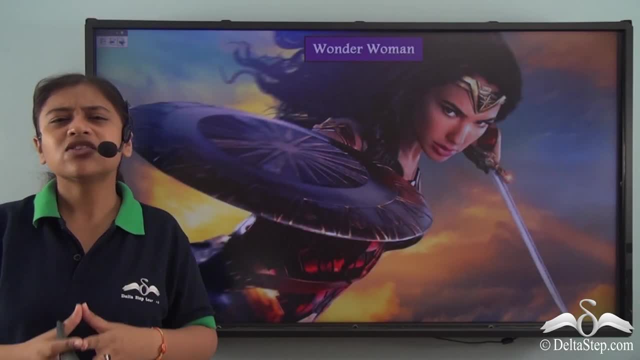 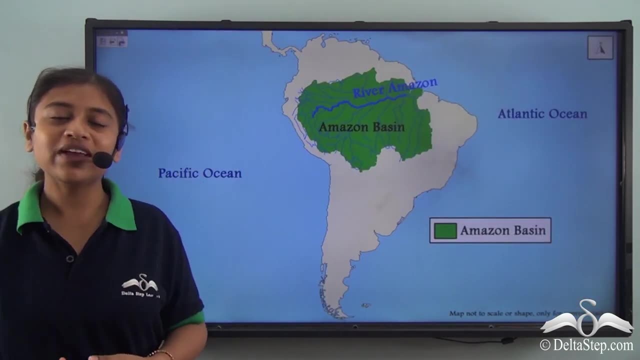 or the conqueror of the lost Amazon river. So now, where exactly do we find this Amazon? Do you know where We find the Amazon? in South America. In our previous lessons, we have been learning about the Amazon basin as one of the most important physical features of the continent And in 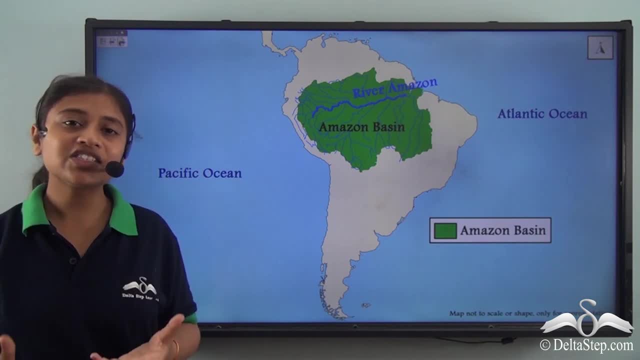 this lesson, we will be learning more about the largest basin on planet earth. It exists as the lungs of the planet, giving out huge amount of oxygen- almost 20% present in the atmosphere- and absorbing large amounts of oxygen. So we will be learning more about. 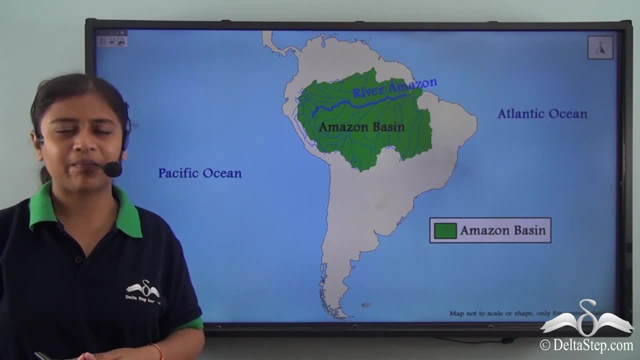 the Amazon basin in South America. It is home to various ecosystems and has a diversified flora and fauna. Now, this basin has a lot of importance and significance when it comes to studying it as a physical feature of the continent. The Amazon basin, as we can see here, expands over or around one of the 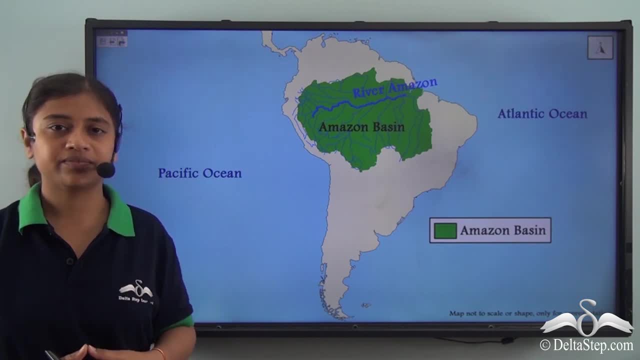 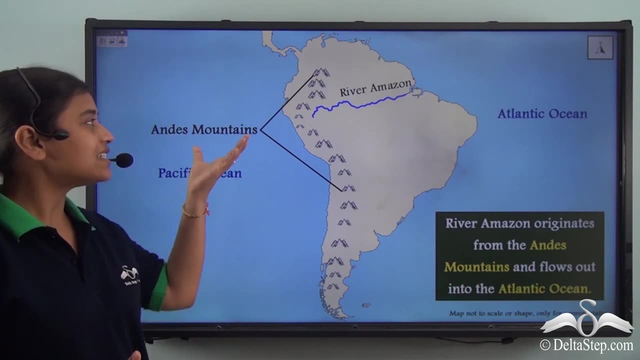 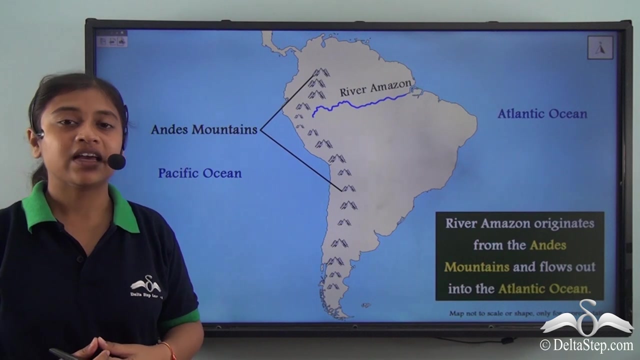 longest rivers of the world, that is river Amazon. Now the Amazon basin. isир point of origin is the Amazon basin because river Amazon originates from the Andes mountains that exist on the western coast of the continent, And we have already learnt this. So it originates in the Andes mountains and it flows out in the Atlantic. 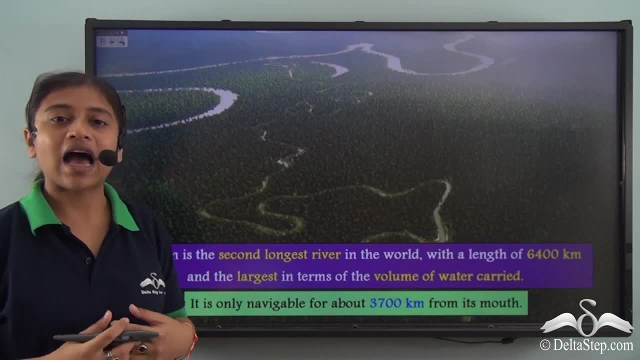 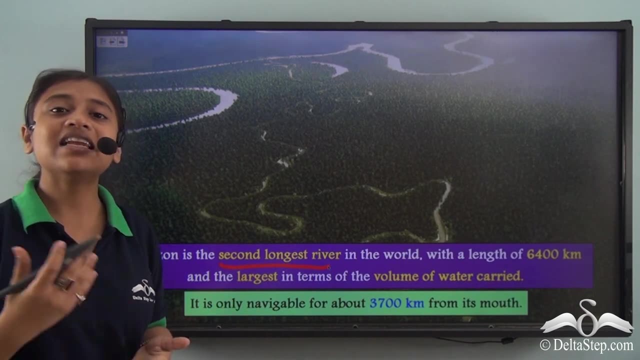 ocean. now the Amazon river is the 2nd longest river in the world after Nile, and it has a length of 6415 m. 2.3 pen. nuestros altos de carekap. Face a 두ên leershirts. after nile, now the Amazon river is the second longest river in the world after Nile, and it has a length of 6400 meters. 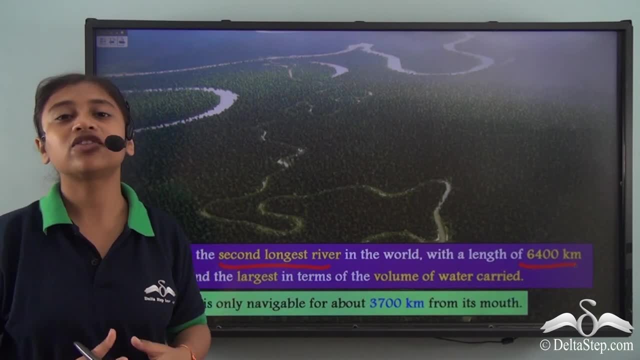 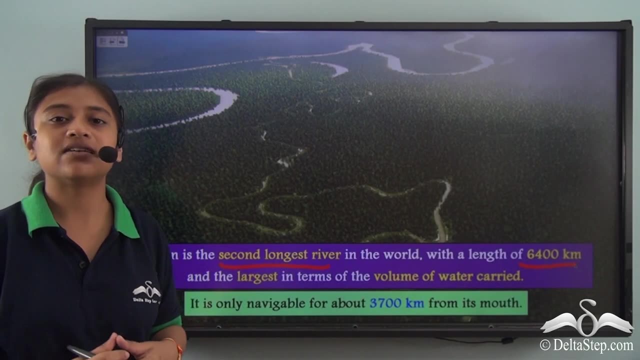 kilometers. Now it is also the largest river of the world in terms of the volume of water it carries. So the Amazon river is the largest in terms of the volume of water carried and the second longest, after river Nile. Now we know that humans are experts and they excel. 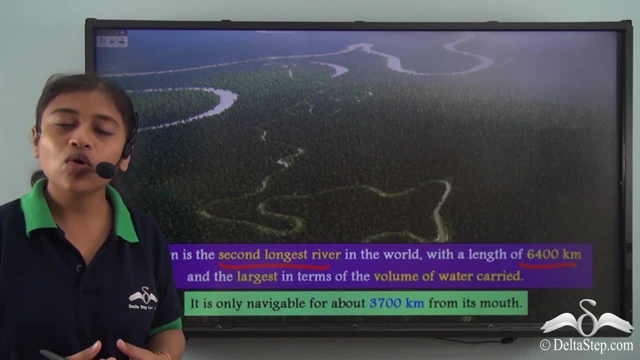 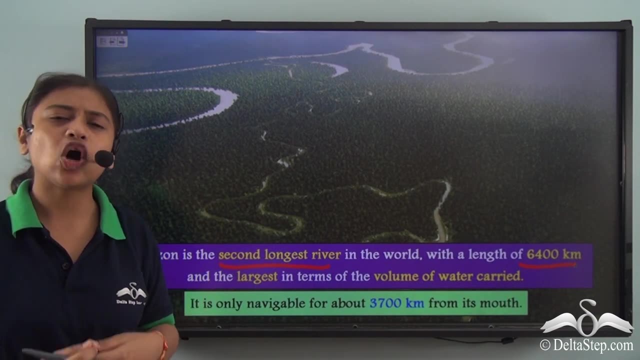 in the field of exploring the mother earth, and so it has done in the case of the Amazon. The Amazon is a living example of where people have not left a chance to explore every minute and every inch of the basin. Now, just like exploring the basin, they have managed to navigate. 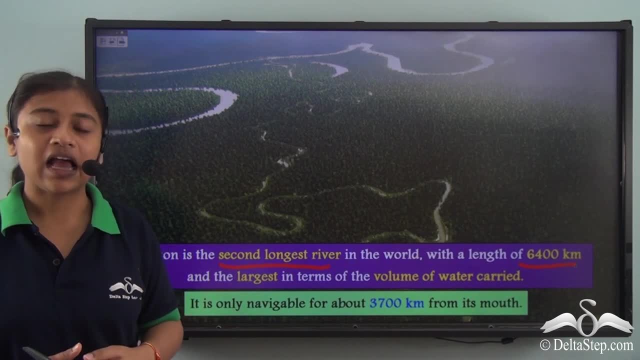 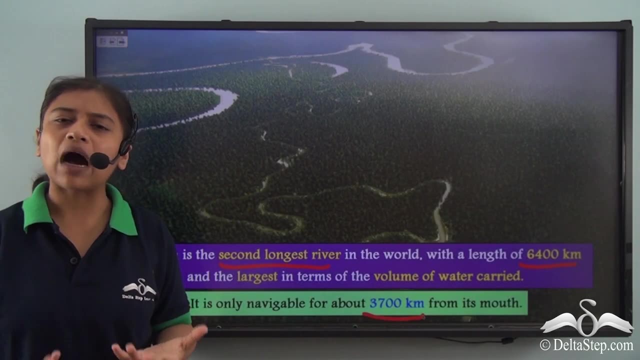 despite difficulties, the second longest river in the world, and they have done that upto a length of 3700 km from its mouth. Now, what is the mouth of a river? So the mouth of the river is where a river joins or flows into a larger water. 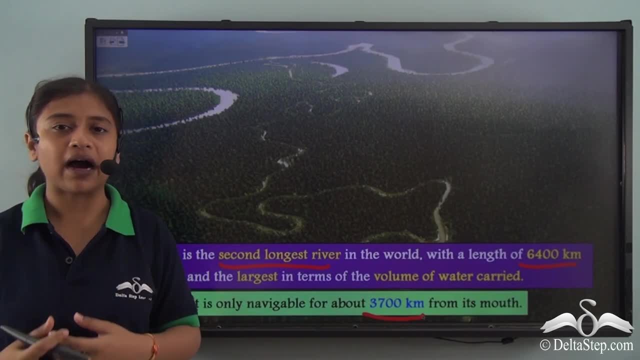 Now, if you want to revise on rivers and its different parts, then you can simply click on the link below and access the iDictionary feature to revise chapters on water bodies. Now let's proceed with a lesson with the Amazon. So here we looked at the second longest river. 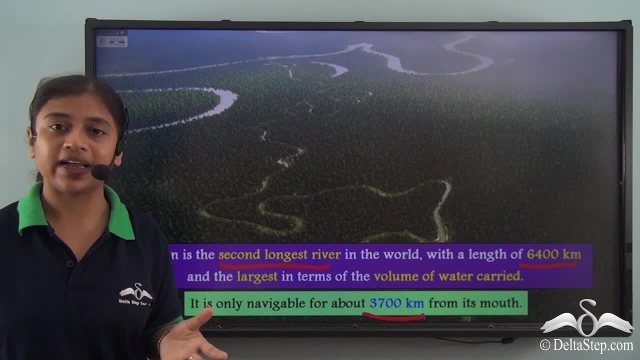 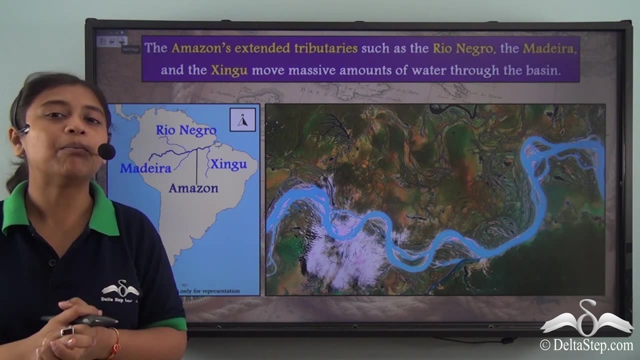 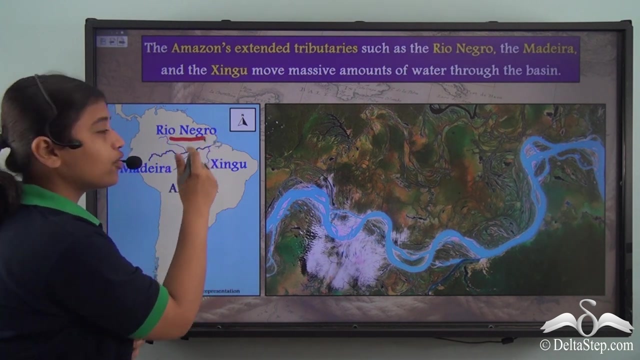 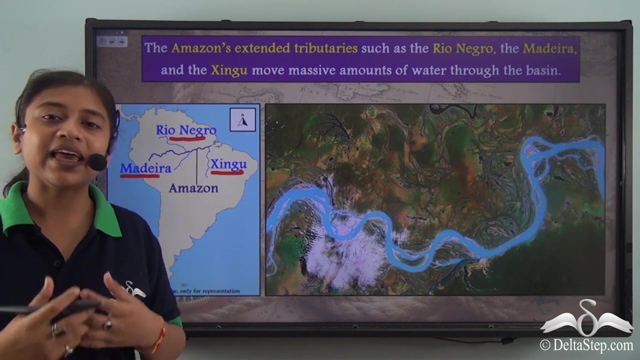 It is also considered to be very, very deep and wide. Now the Amazon's extended tributaries play a very important role in the Amazon basin. The extended tributaries include Rio Negro in the north, Zingu and Madeira. Now these trees are the major tributaries that join the Amazon river and flow over the. 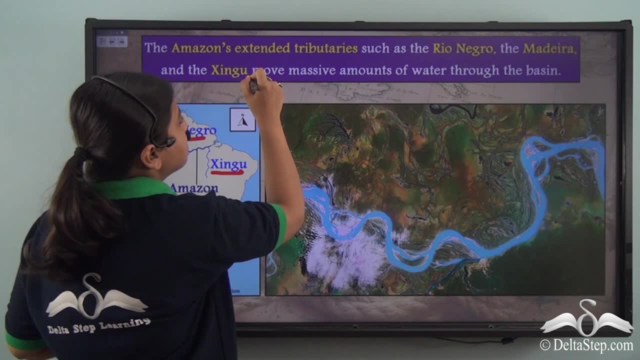 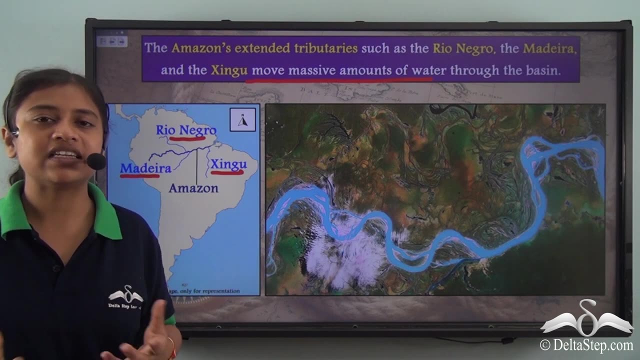 Amazon basin. They tend to move massive amounts of water through the basin, Thus making it very, very rich and fertile in nature. Now, other than these, it is estimated that around 1100 other tributaries are a part of the Amazon river system. 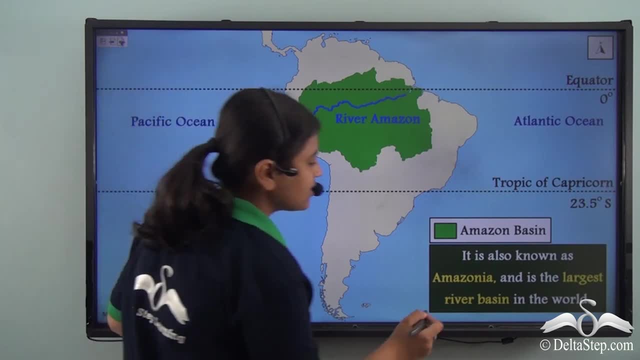 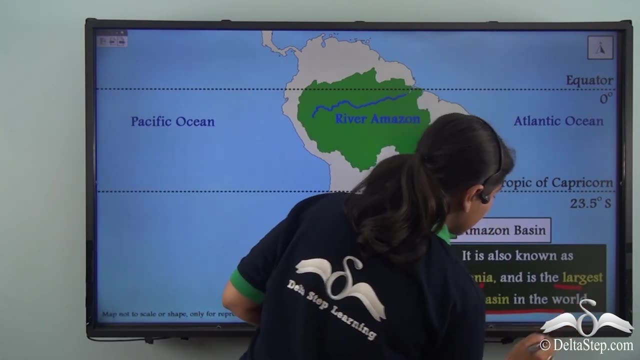 The Amazon river basin is also famously known as the Amazonia and, as I mentioned earlier, it is the largest river basin in the world. Let us look at the latitudinal extension. Let us look at the latitudinal extension. Let us look at the latitudinal extension. 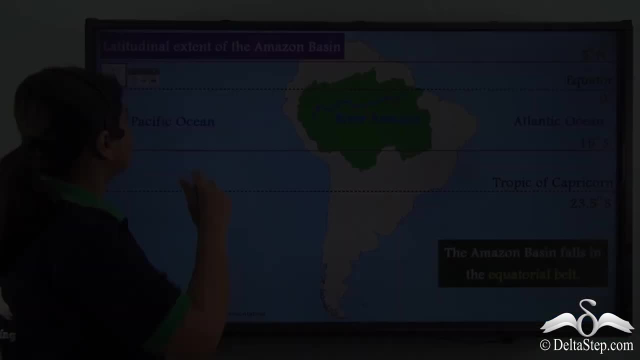 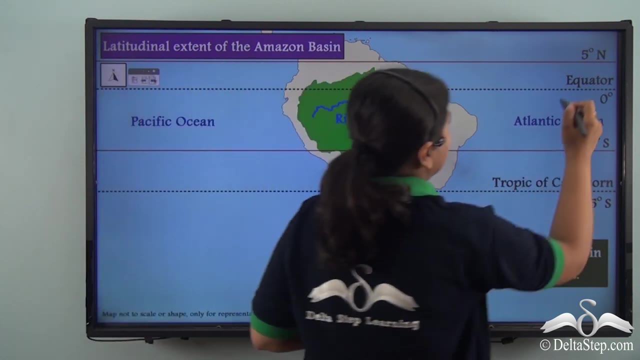 So what is the relation to the west? They are instead the easternmost kardeşim Territory, If you understand, represents the position of Laser beam. So, as we have already learnt in our previous lesson, the Amazon basin extends from 5 degree. 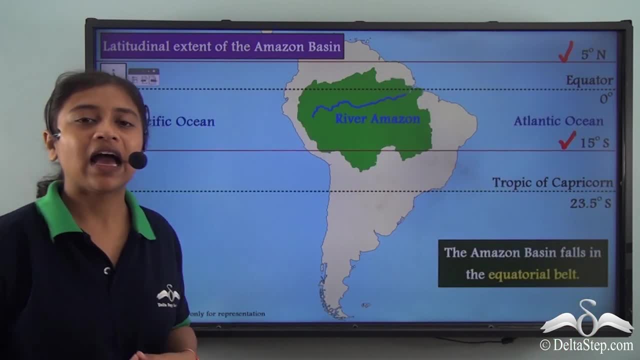 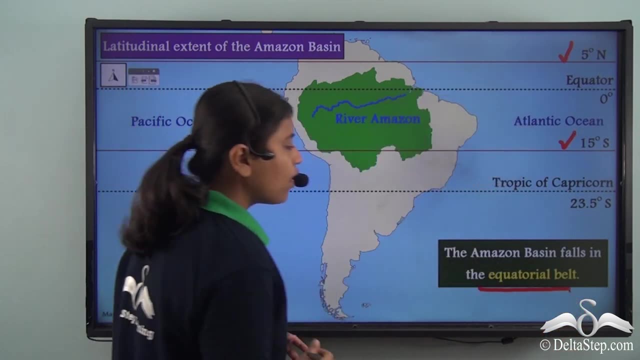 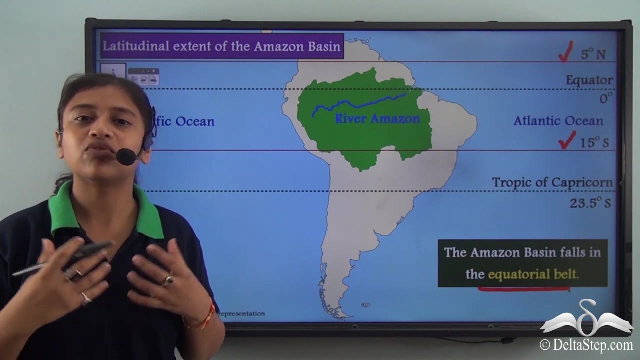 north to 15 degree south latitude, and thus we can see that it mostly lies in the equatorial belt, that is, around the equator. Now, what does tell us This? tells us that, following in the equatorial belt, it experiences rain almost throughout the year, and this organisation is due to Prozent d. 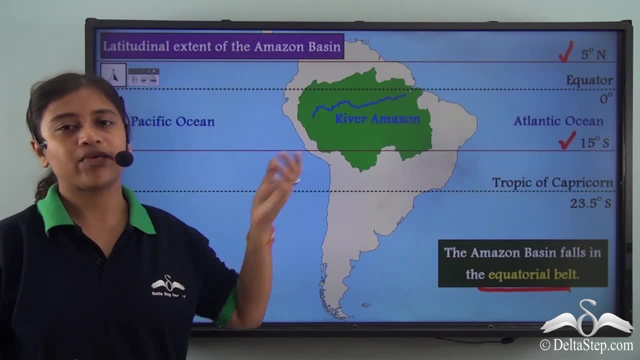 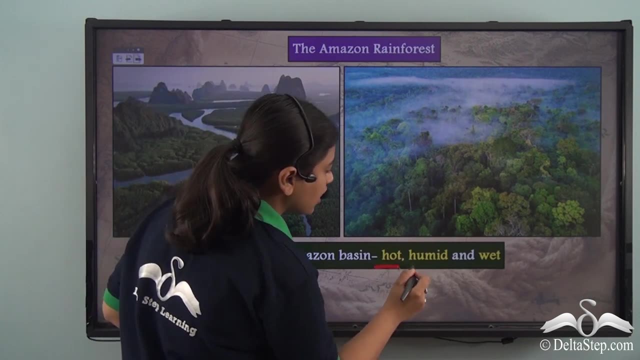 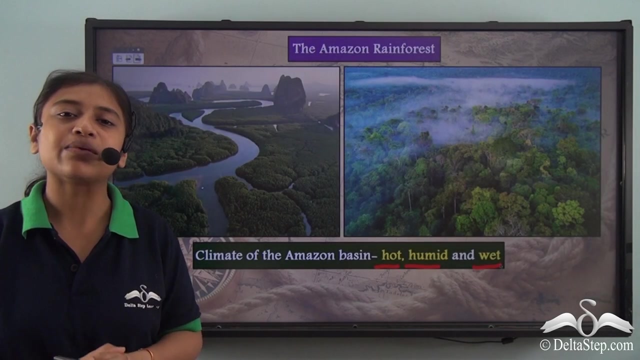 and thus it is also known as evergreen forest. So, as per the climate of the Amazon forest, it is hot, humid and wet. This is same as the other key characteristics of the places that lie in the equatorial belt. So it experiences. 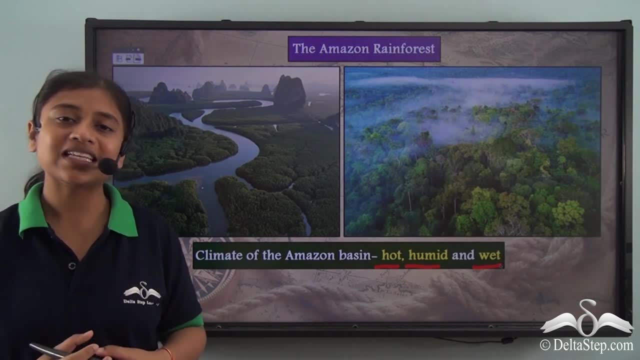 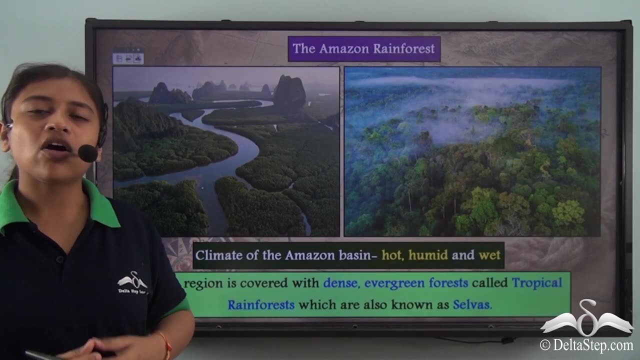 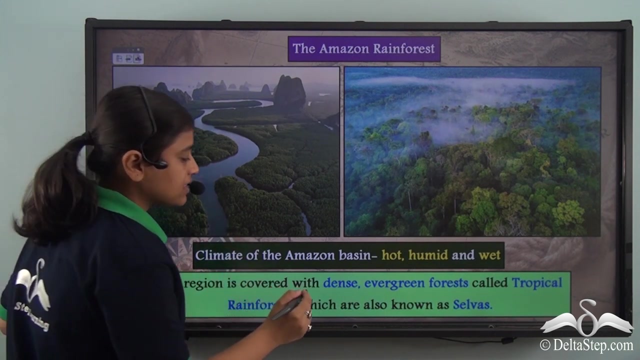 rain throughout the year, it is moist, humid, wet, and it is also hot, as it receives direct rays of the Sun almost 24-7.. Now, because of this unique climate, the region is covered by thick, dense forest, So the Amazon basin is covered by. 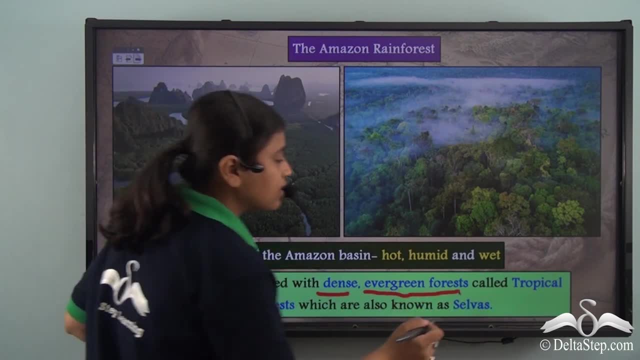 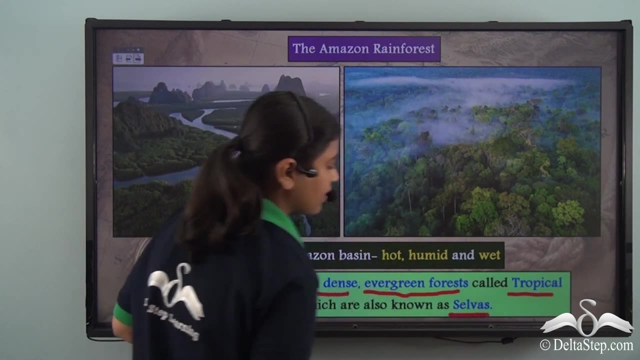 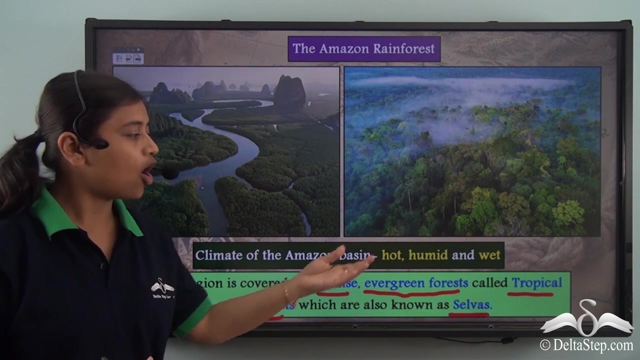 dense evergreen forest, and these are called the tropical rainforest. Now these are also known as Selvas. So we understood that the Amazon basin, since lies in the equatorial belt, experiences a hot, humid and wet climate, because of which the region is entirely covered by. 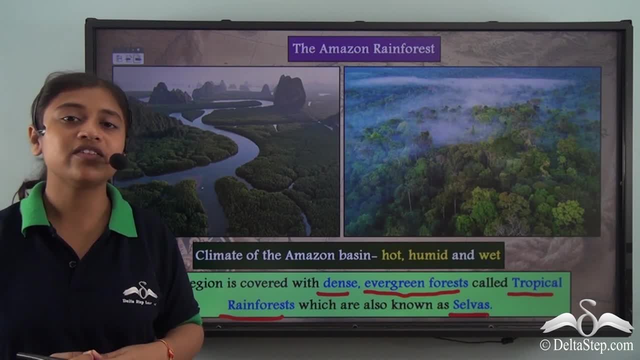 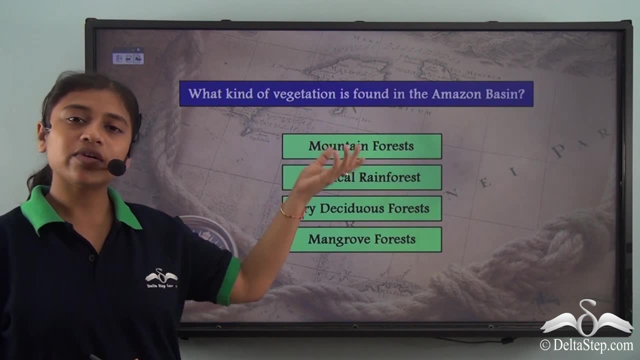 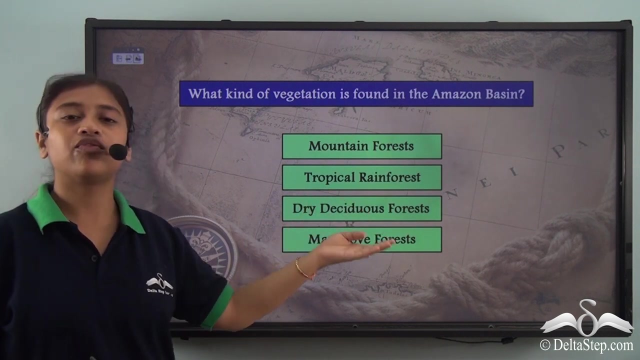 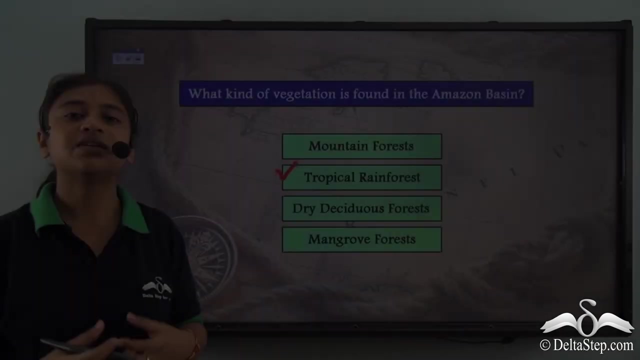 dense, thick, evergreen forest, known as tropical rainforest and also known as Selvas. Do we find their mountain forest or tropical forest, or dry, deciduous forest, or do we find their mangrove forest? Yes, we find tropical rainforests as the most prominent vegetation of the Amazon basin, The Amazon rainforest. 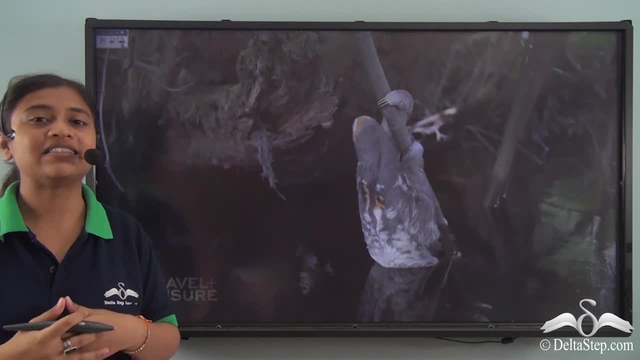 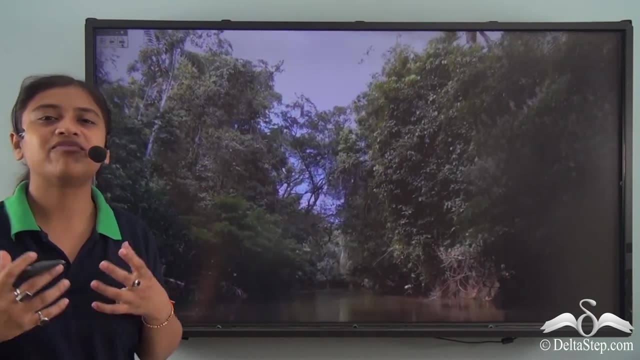 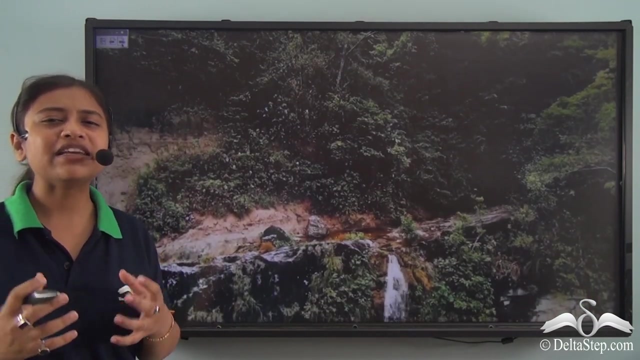 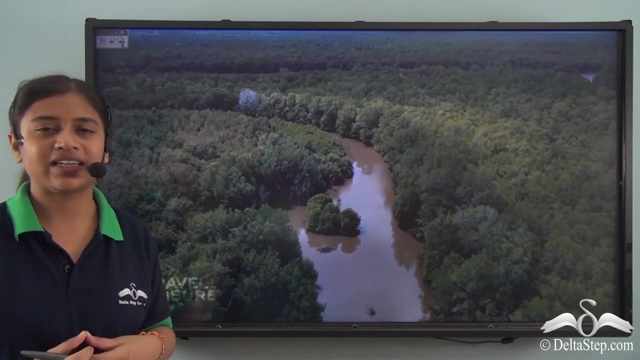 that exists on the Amazon basin is unique and diverse, both for its flora and fauna. The flora& fauna here has a species, a variety of which includes different animals and plants. The region is also known for magnificent and beautiful waterfalls, different water bodies, seasonally flooded savannahs and wetlands. 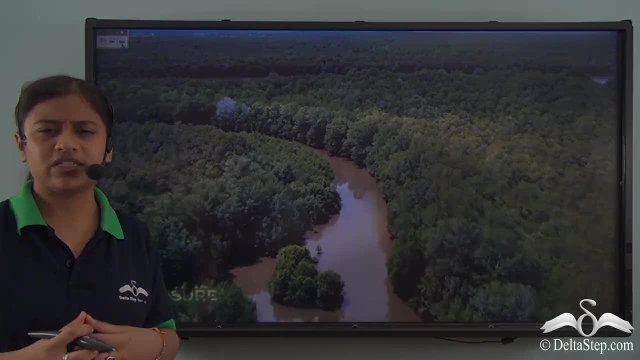 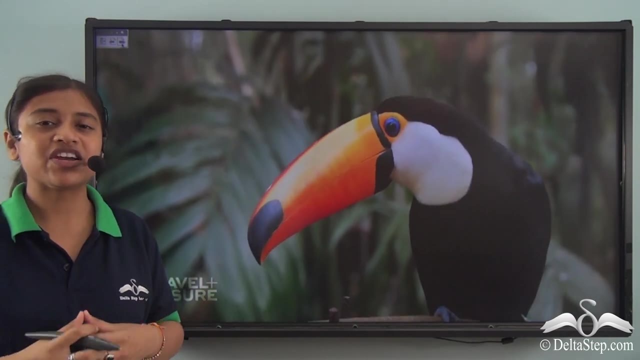 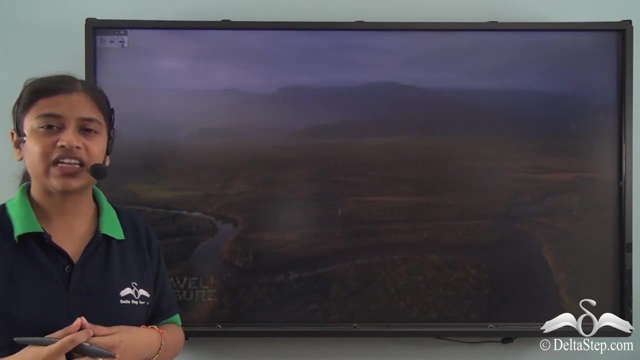 The region here is covered by thick, dense forest that forms a roof like structure by its leaves that does not let the sunlight penetrate and reach the ground, leaving the ground damp and dark Now, because of which the region is rich in trees that are shade tolerant. 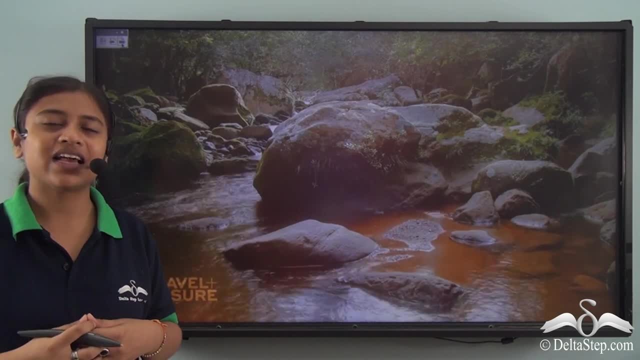 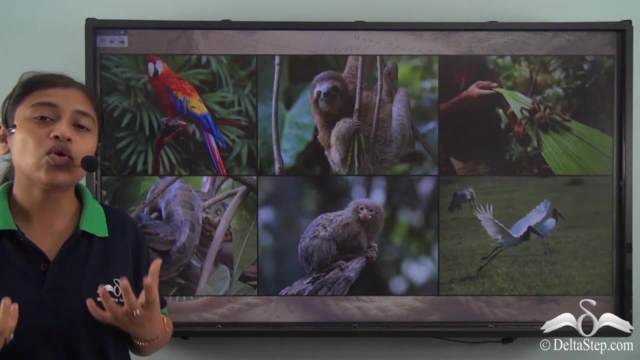 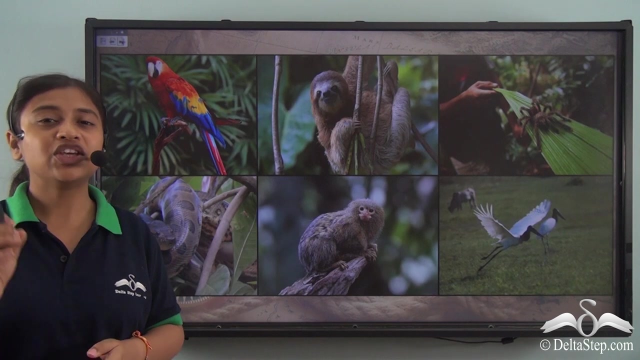 So the Amazon basin is unique in its own and it acts as the lungs of the earth. With such rich flora, the region is known for a unique fauna. We have already discussed in our previous lesson about some of the most unique animals that we see there, like the capybara, tapirs, squirrel monkeys, owl, butterflies and many. 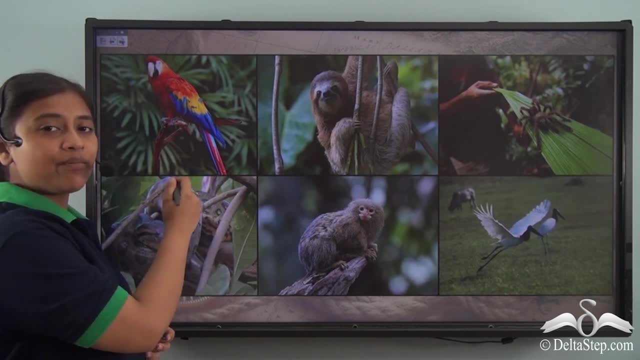 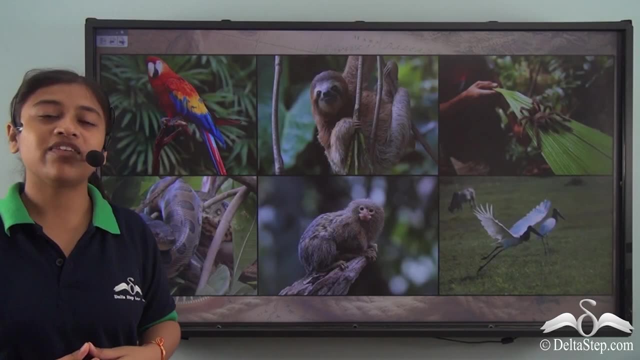 more. Here are some more of them. We have Macau sloths. We also have the largest species of spiders, that is the goliath spider. Here we also find some of the largest snake species, that is, the anaconda. You must have heard and seen movies about anaconda. they are large and they are very 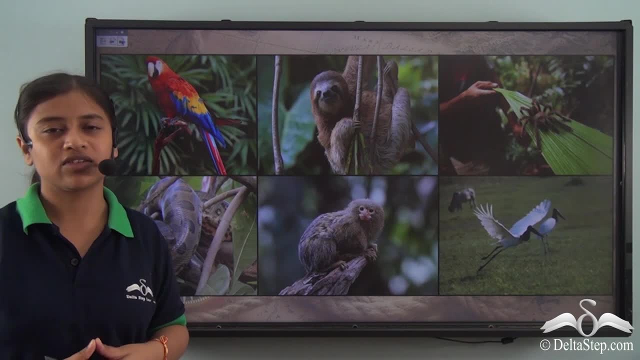 dangerous. We find such unique animals only in the Amazon. We also find here some of the smallest types of monkeys, and they are known as mermosats. On the other hand, we also have some of the most significantly beautiful animals. We find some of the most beautiful birds, like the storks. 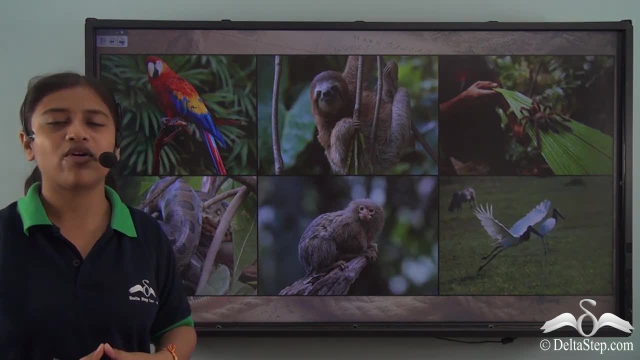 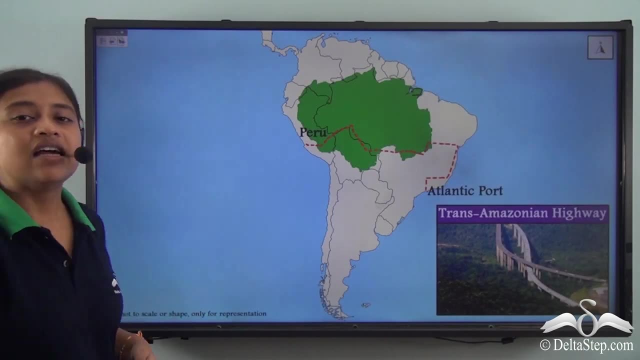 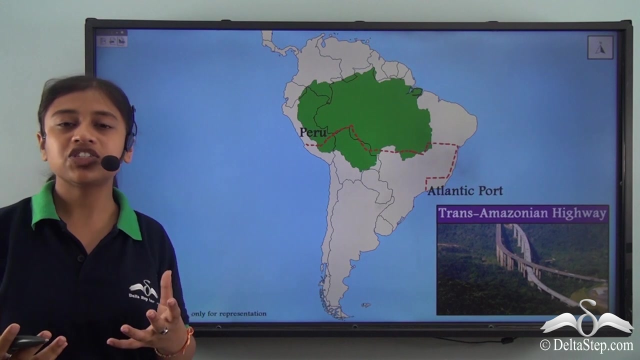 So you see that the unique basin and the largest rainforest is aptly called unique because of such varied plants and animals. Now, as I have been mentioning, the forest here is very dense and thick, So penetrating and researching about the different flora and fauna was very difficult for the 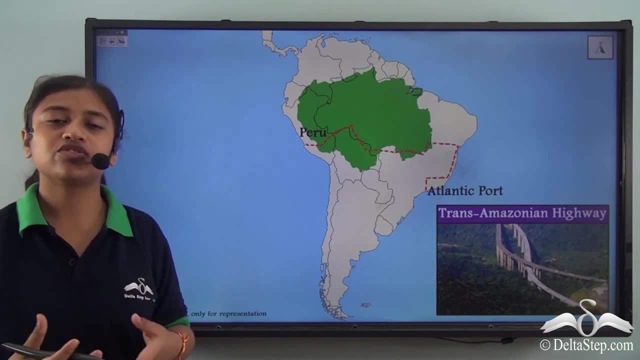 scientists in the earlier times. However, over the years, due to advanced technologies and access to different species of animals, we have been able to find some of the most beautiful birds, like the storks. So you see that the unique basin and the largest rain forest is aptly called unique because 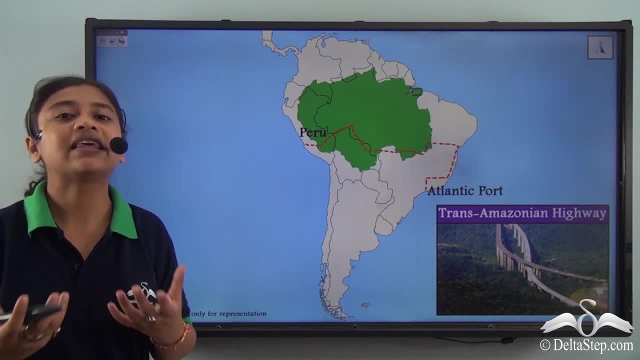 of such varied plants and animals. Now, as I have been mentioning, the forest here is very dense and thick, So penetrating and researching about the different flora and fauna was very difficult for the scientists in the earlier times. So penetrating and researching about the different flora and fauna was very difficult for the 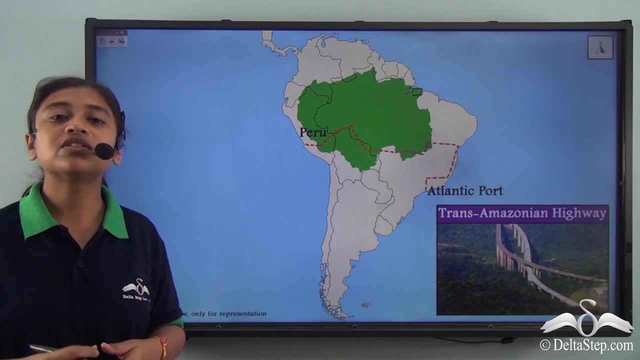 scientists in the earlier times. However, over the years, due to advanced technologies and access to different machines, now the research are being carried out with the help of helicopters and drones. Now, over the years, one of the most important developments in South America has been the. 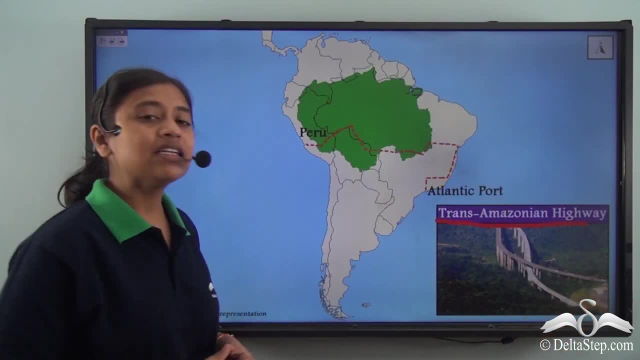 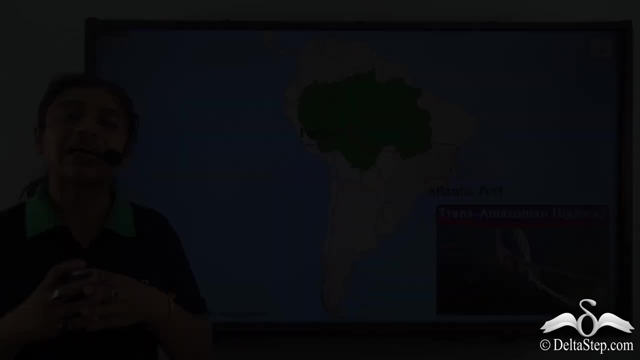 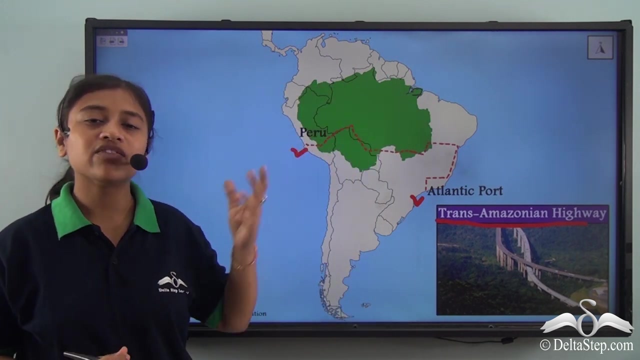 Trans Amazonian Highway. Now, the Trans Amazonian Highway is the only highway that crosses through the thick Amazon forest, connecting the Peru coast with the Atlantic port. It is one of the longest highways of the world And it is the only highway that cuts through the thick Amazon basin. 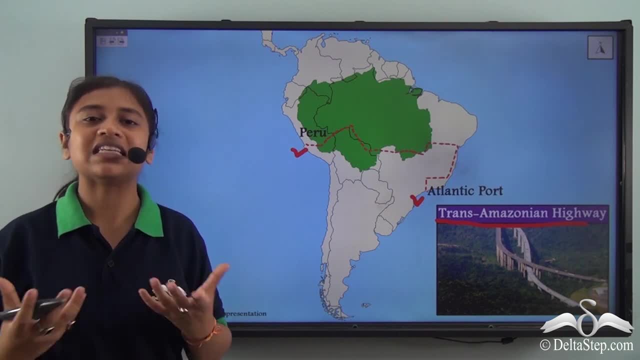 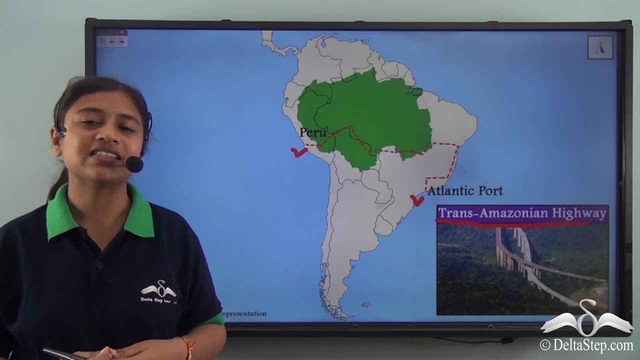 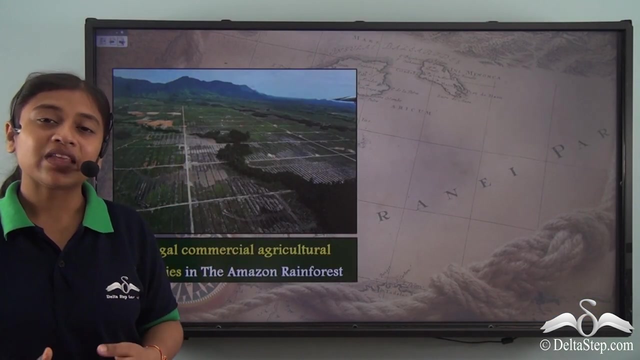 Now, this particular highway has also made access to this forest easier, thus helping the scientists and researchers to explore more undiscovered and unrecognized species that exist in the Amazon forest. Now, as the global time is proceeding, the demand of the growing population is also to 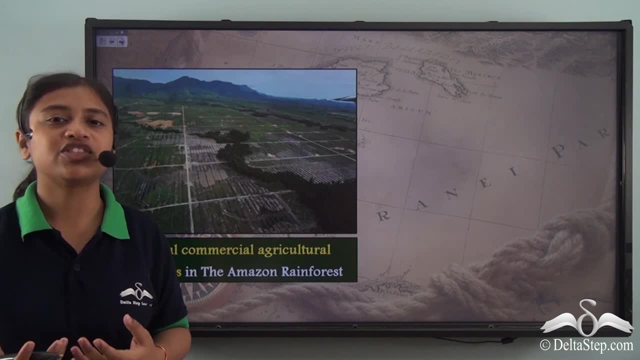 be met And only to do that. the Amazon is being misused. There are various. There are various. There are various illegal commercial agricultural activities that are carried out in the Amazon basin. We know that the Amazon absorbs large amount of carbon dioxide. 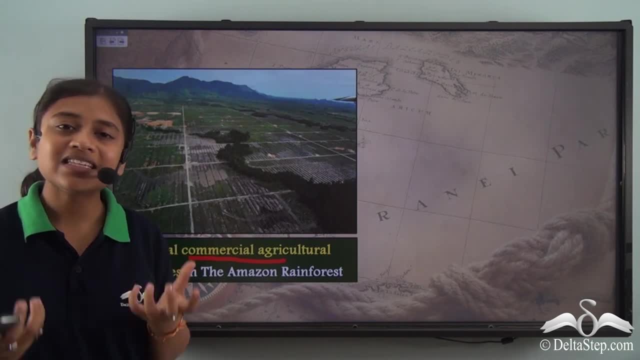 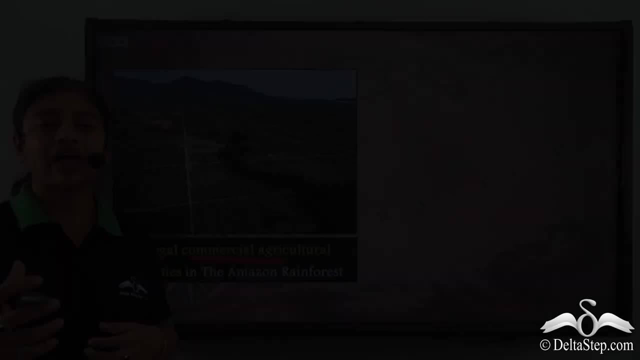 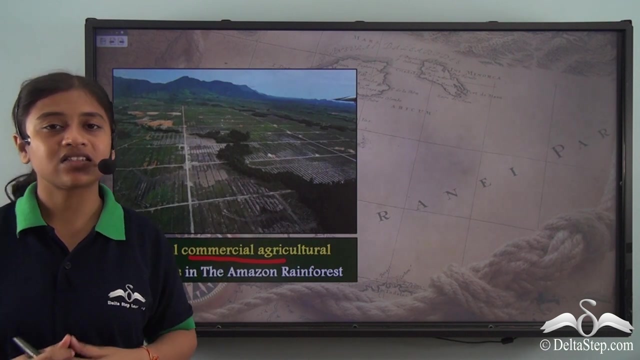 When the same forest is being cut down, the carbon dioxide that exists in these trees tend to escape into the atmosphere, thus increasing the overall temperature of the earth and adding to global warming. So the human activities are the key cause of losing such beautiful wonders that exist. 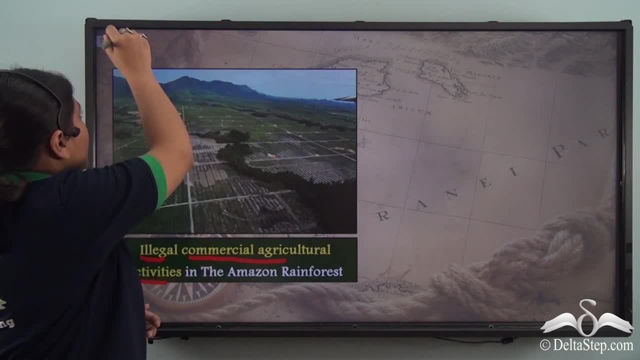 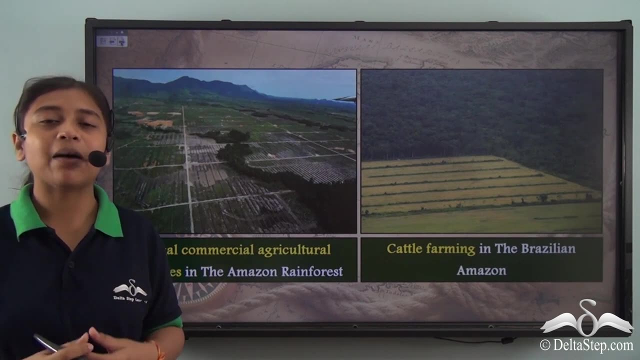 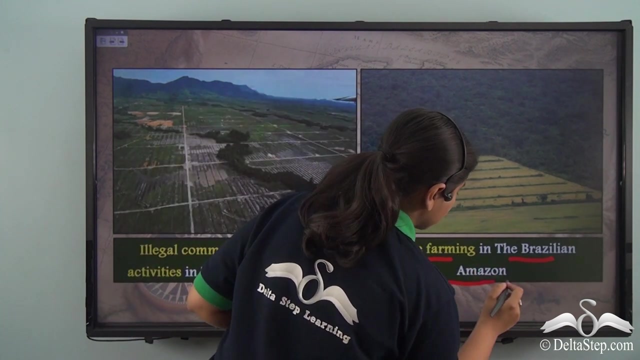 now, but it might not later. Now, other than the illegal agricultural activities, we also see clearance of vast areas of the Amazon basin for cattle rearing and cattle farming, especially in the Brazilian Amazon. Now Brazil is one of the countries that have been warned by international community to 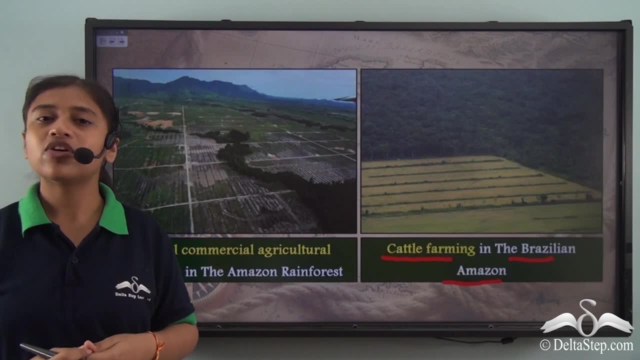 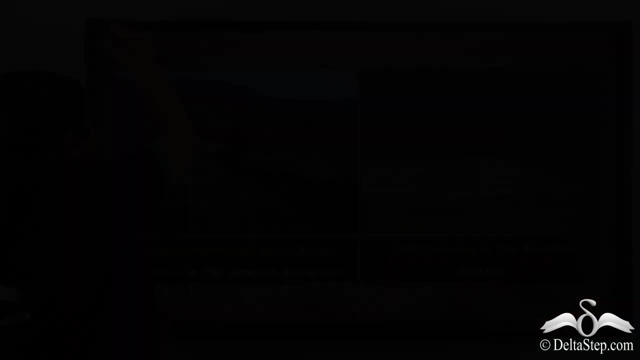 cut down on the deforestation, because we need to realize the deforestation of the Amazon will not only harm the forest, But the deforestation of the Amazon will not only harm the forest, It will harm the entire humanity that exists today. When that wasn't enough, people had no less greed and they carried on with their illegal 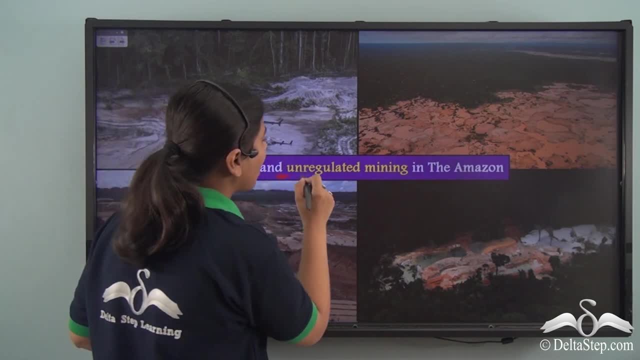 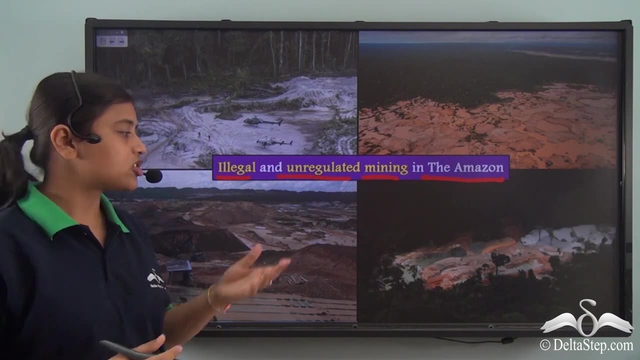 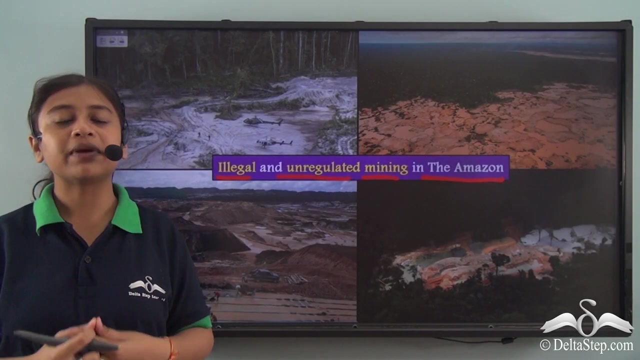 practices, which also included illegal and unregulated mining in the Amazon. Now, this not only is destroying the vegetation of the place, but also the soil that holds on to the vegetation, thus leading to the overall degradation of the very important and significant basin on earth. 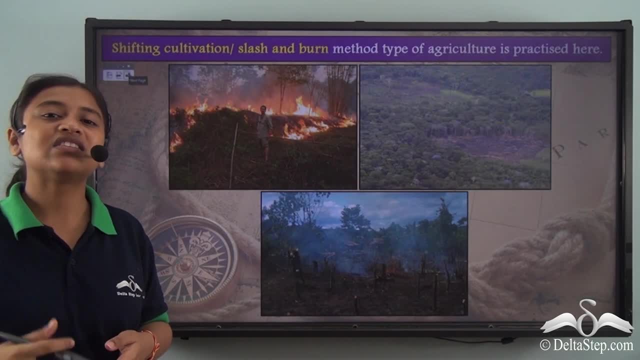 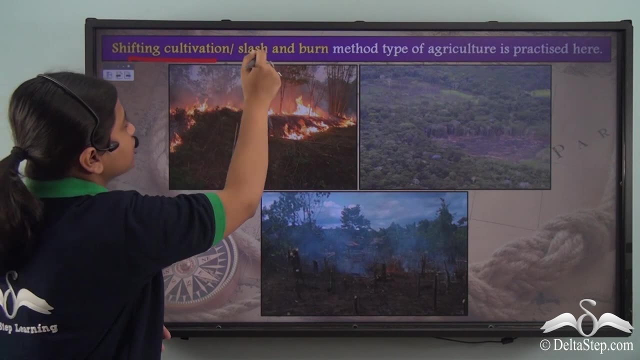 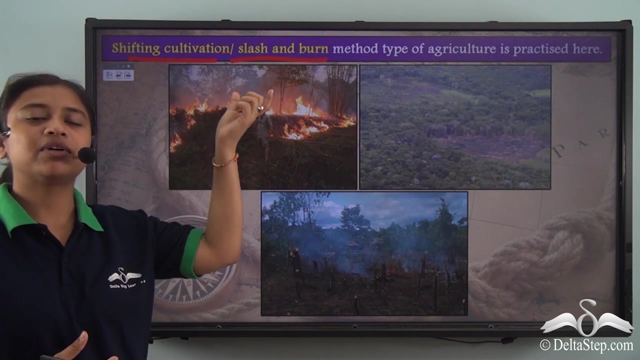 Now, another important factor that has led to the degradation of the soil and the vegetation of the Amazon is the traditionally used shifting cultivation or slash and burn method of agriculture. Now, firstly, what exactly is shifting cultivation or slash and burn agriculture? It refers to that type of 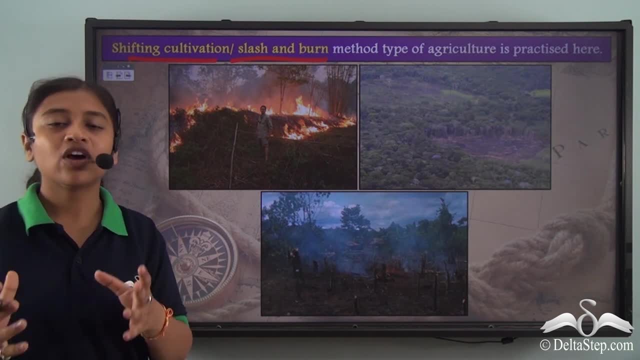 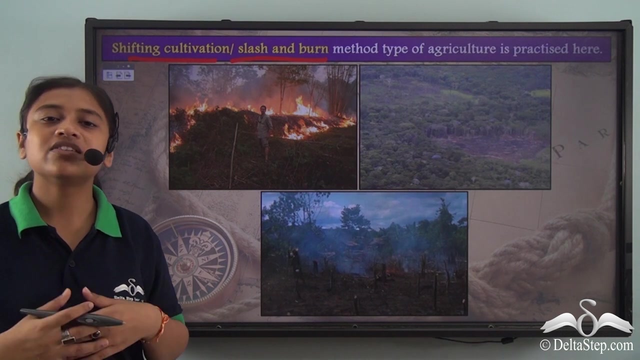 agriculture, where people clear a plot of land, grow crops there, that is, they cultivate that land and over the years, when that land has lost its fertility, they move to another piece of land, clear it, burn the land and then repeat the entire process. So you see, 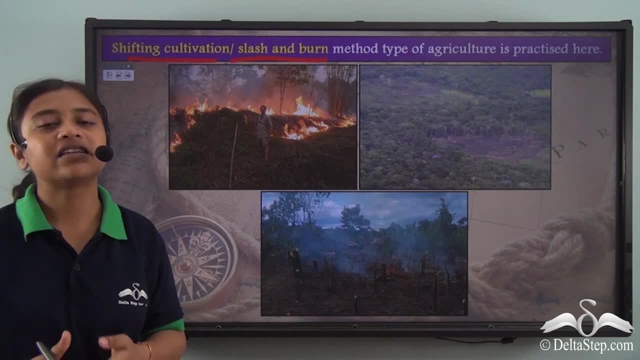 they slash out the trees, burn the land and cultivate the land. This is one of the most primitive methods of agriculture that has been used in the ancient times and it is still prevalent in the Amazon, So it has played a very important role in destroying 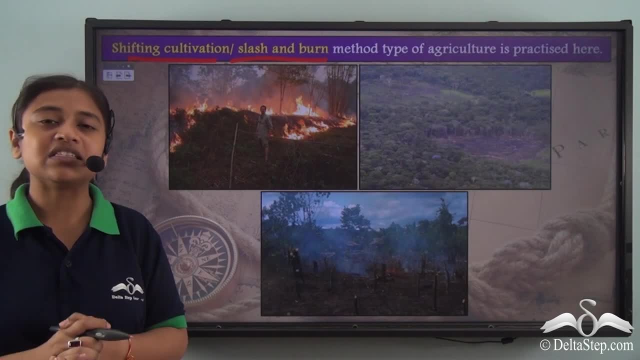 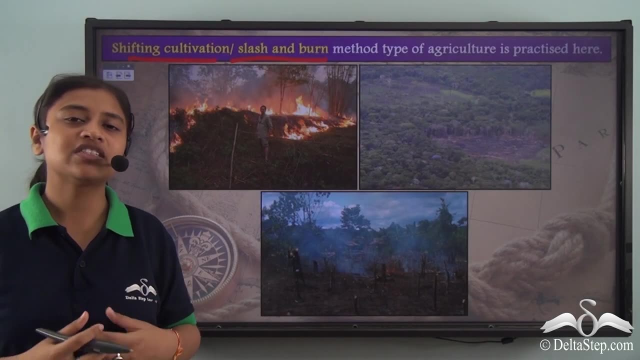 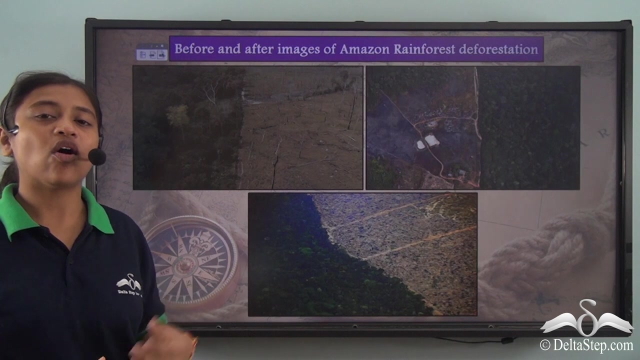 the ecosystem that exists in the Amazon. It has led to the degradation of the soil, making it very, very unfertile, and it also has harmed the beauty of the magnificent Amazon. Now it's quite unfortunate to see the before and after images of the Amazon rainforest. 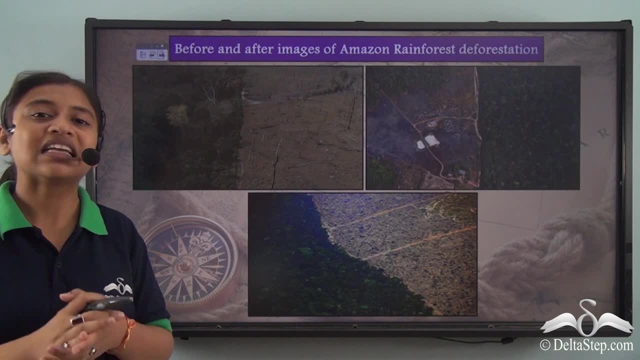 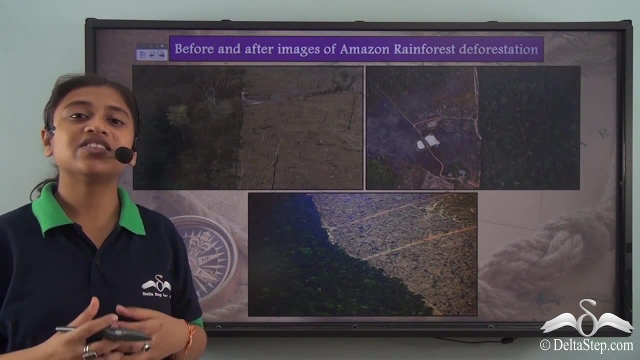 We see that large areas of the land has been cleared for agricultural purpose and for cattle rearing. It will be too late to realize that the Amazon is the resource that we can use in our fight against global warming. It will actually cease to exist and will turn out to be very bad for the future generation. 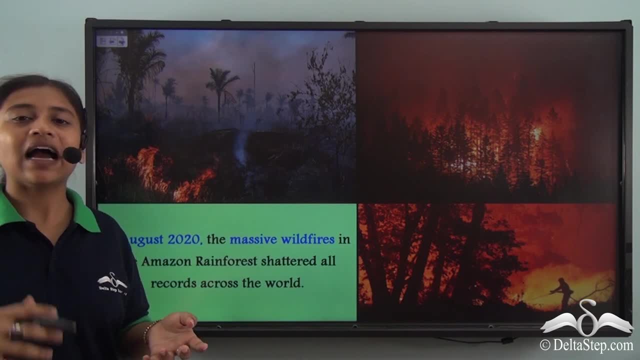 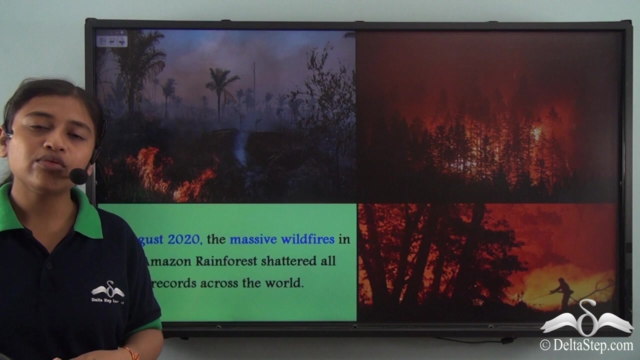 Now, because of various agricultural activities, both legal and illegal. the region has suffered a lot of climate change. The climate over the Amazon is believed to be drying out Now. because of the climate drying out over the Amazon, it has left the forest vulnerable to drought and forest fires. The wildfires have been worst in 2020, especially in the month of August, where Amazon faced severe and threatening wildfires that shattered all records of the world. Agriculture practices, particularly the slash and burn method of agriculture, has been responsible for different wildfires in the Amazon. Now these wildfires have extended to unintended places and for which 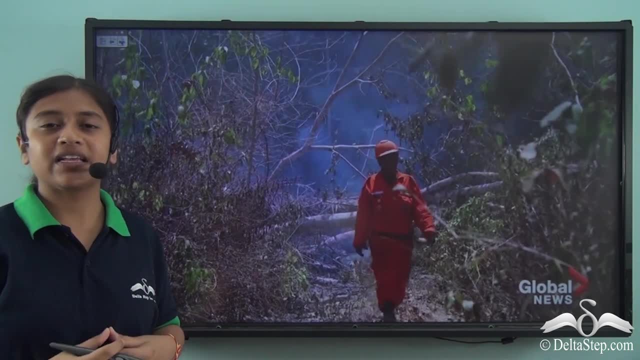 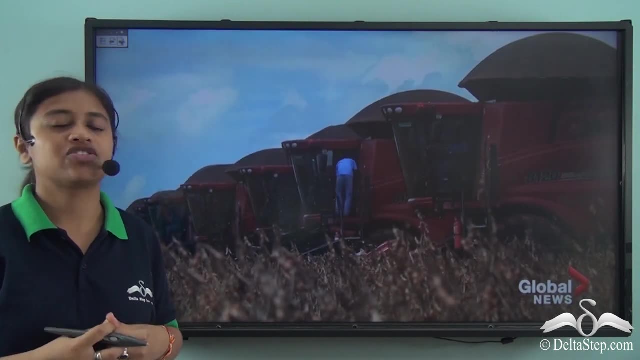 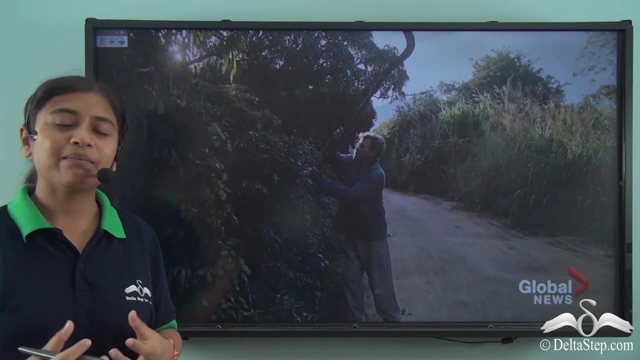 people were not prepared. Though the locals say that farming is a primary activity and they are economically dependent on it, they need to be careful on how they carry on with their agricultural activities. The Amazon has been vulnerable to such wildfires and drought. The region or the climate over the Amazon? 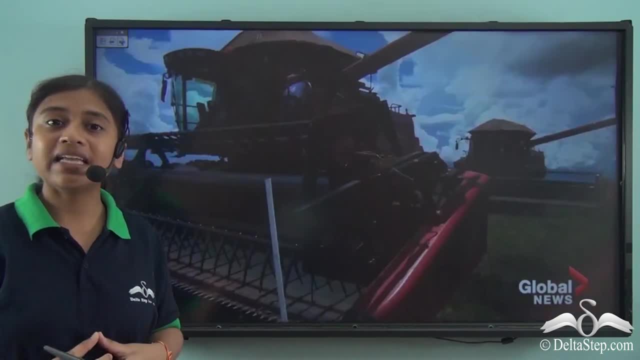 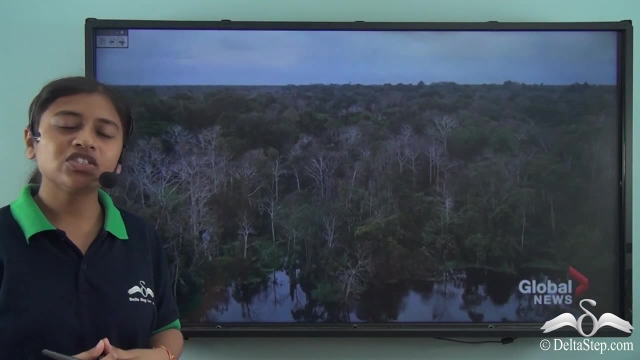 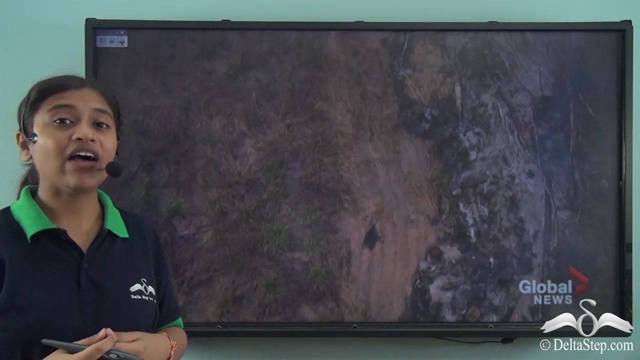 is drying out, and it is a matter of concern. It is believed that the Amazon is emitting more amount of carbon dioxide than it is absorbing it, and the oxygen level that it used to provide us with is actually decreasing day by day. Now we need to understand that we have the opportunity of using Amazon as a resource. 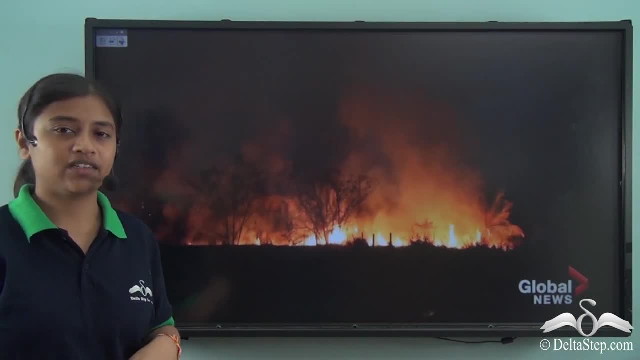 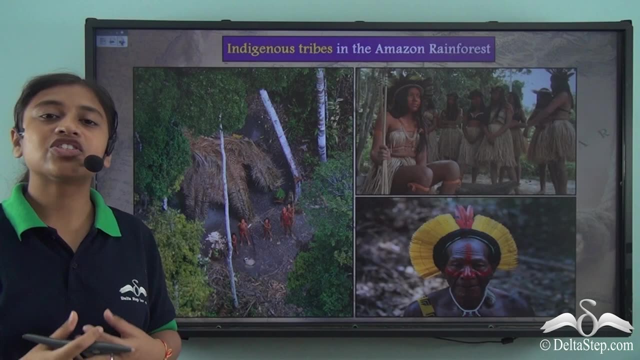 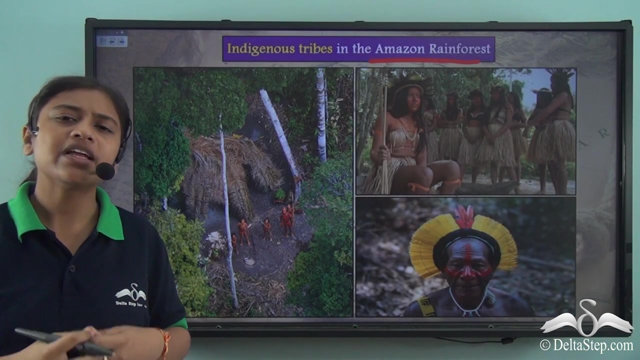 in our fight against global warming, rather than destroying it. Deforestation and other such illegal practices like mining have destroyed the lives of indigenous tribal people living in the Amazon rainforest. They have been living here since the prehistoric times. They are completely dependent on the rainforest, So if we, only for our greedy needs, cut down. 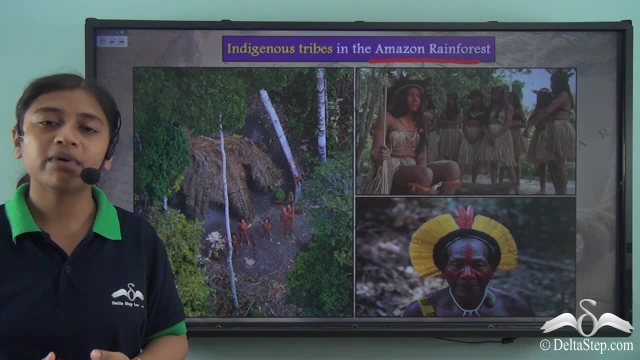 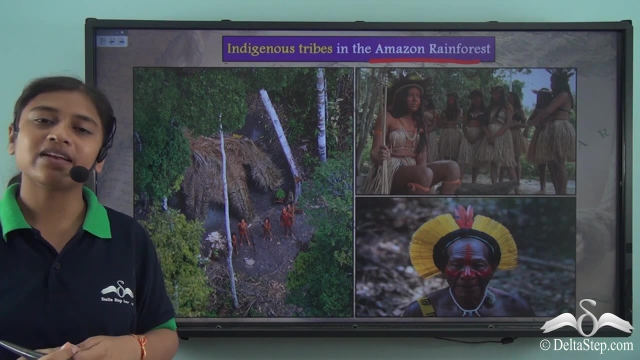 on these rainforests, then it will not only take away their home but also kill them, as they are not ready for the modern world, They are not exposed to the modern world and they are only dependent to the primitive methods of living. So measures need to be taken in. 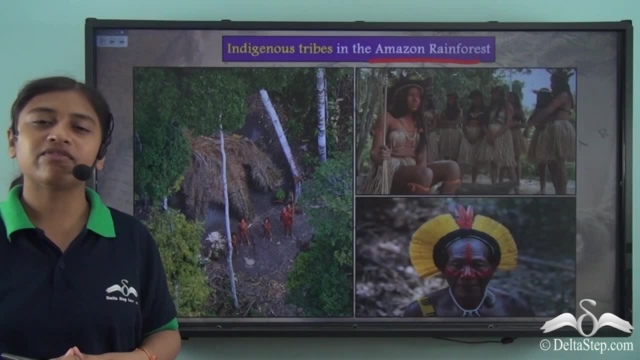 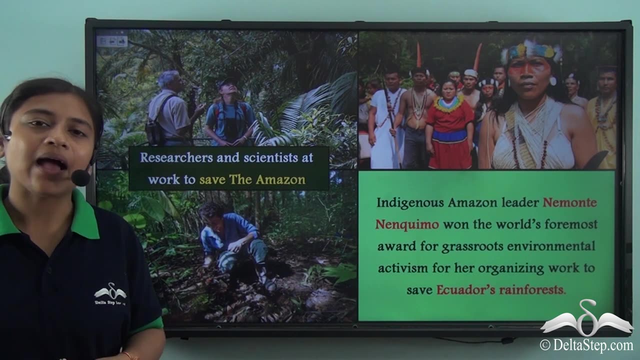 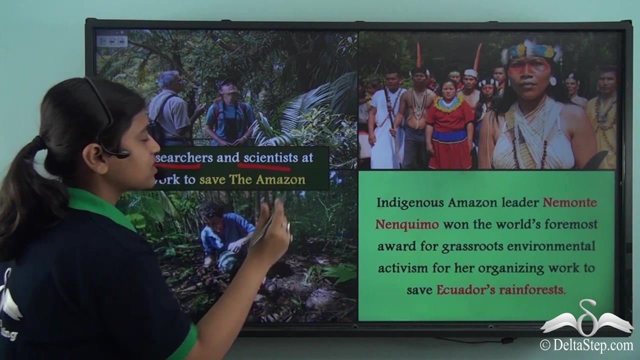 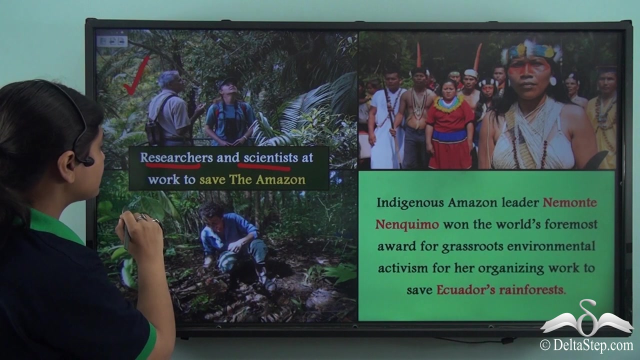 not only by the countries of South America but globally, to save what is known as the magnificent Amazon. With environmental awareness and camps being carried out at various places across the globe, there are various researchers and scientists working hard to conserve and preserve the Amazon. We can see pictures here where researchers and scientists are working hard to save the. 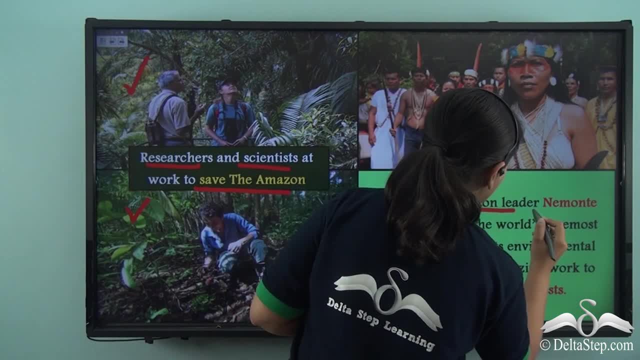 Amazon. Now, a very good example of this same is of the indigenous Amazon leader, Nemonte Nenqemo. There he was fighting for the safe next to home. People used to say that it could be the mother of abekham Himself who moves the wavelength. 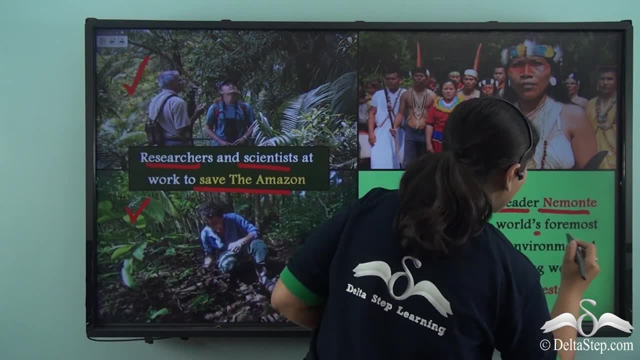 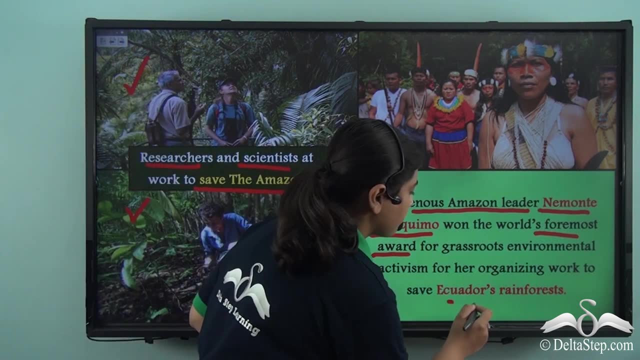 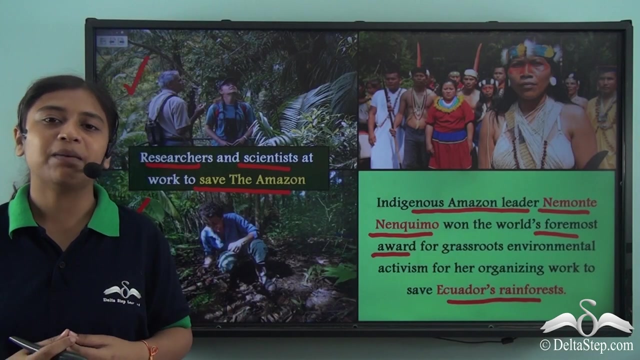 He potentiallyors his sentenced to lilac if he is serving a thane language- In fact one of her. She won the world's foremost award for grassroot environmental activism to save Ecuador's rainforest. So, just like her, we all can take little steps to save our Amazon and the nature with which we are blessed. 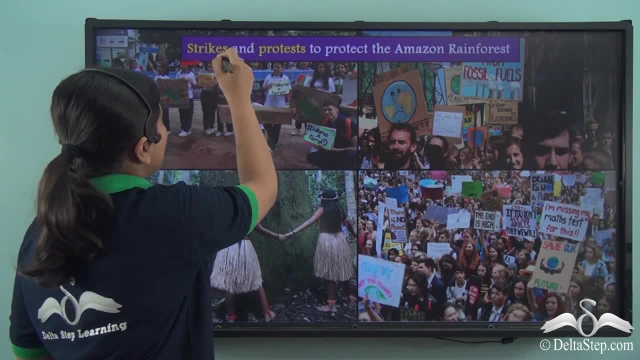 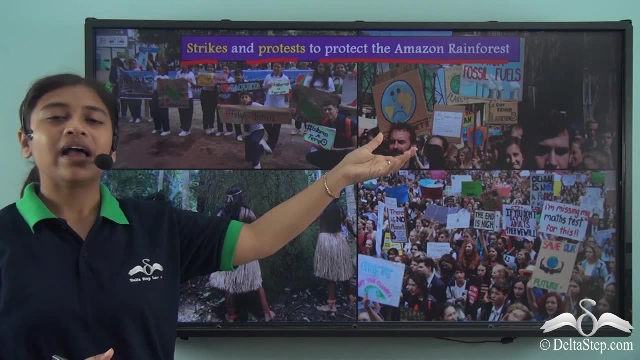 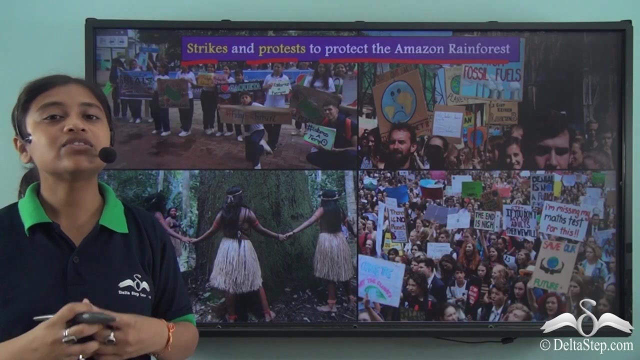 As part of the awareness, there are various strikes and protests being carried out to protect the Amazon rainforest. We can see here people from across the globe carrying different play cards, painting their faces, going on rallies, sitting down on strikes and protests only to save the Amazon.